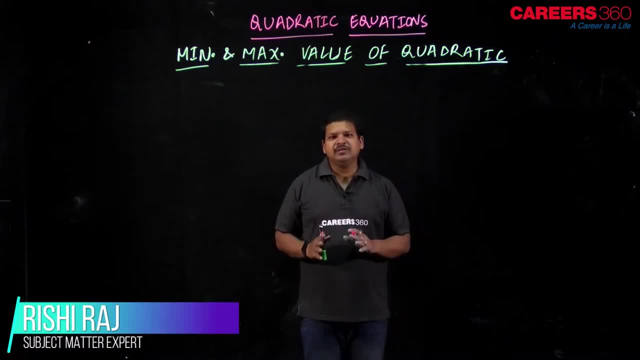 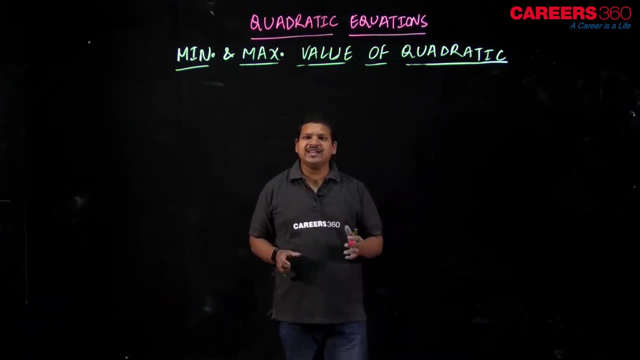 Welcome back everyone. So we are going to understand in this session the minimum and maximum value of a quadratic. Firstly, you need to understand the mathematical derivation of how we can get the minimum and maximum value of a quadratic, and then I will let you understand the. 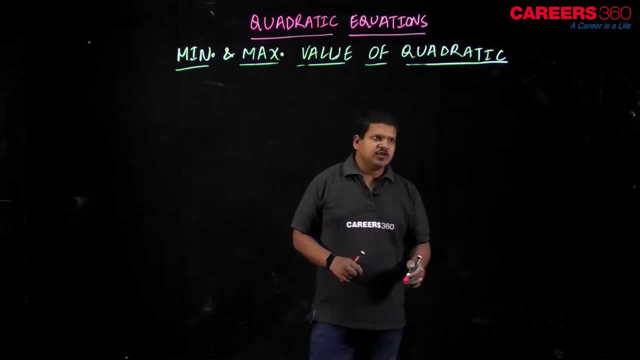 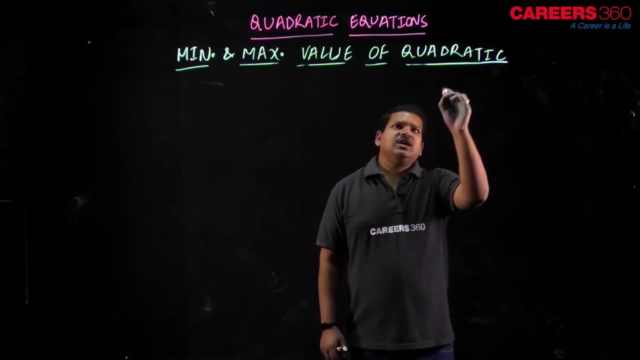 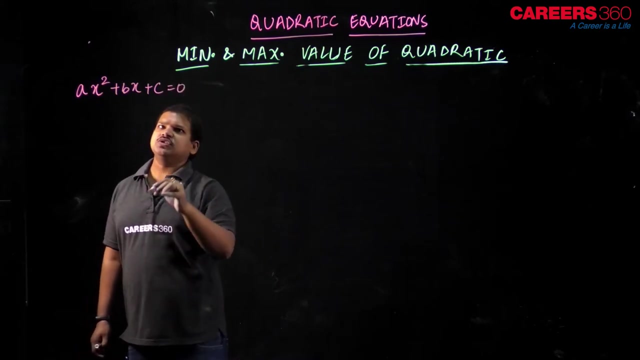 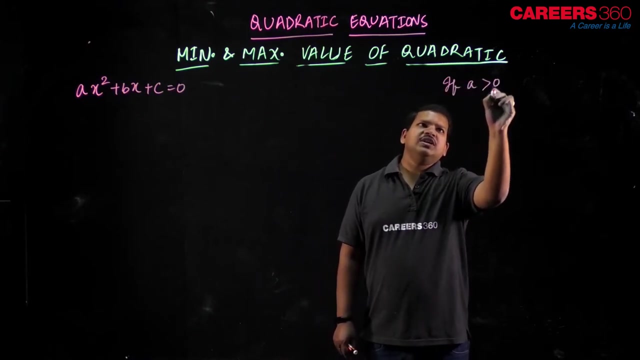 graphical representation of this as well. Firstly, there is this basic thing with respect to graph that you need to understand, that is, let us say there is this equation: Ax square plus Bx plus C is equal to 0, right, and let us say, if A is positive, if A is greater than 0, right? So if 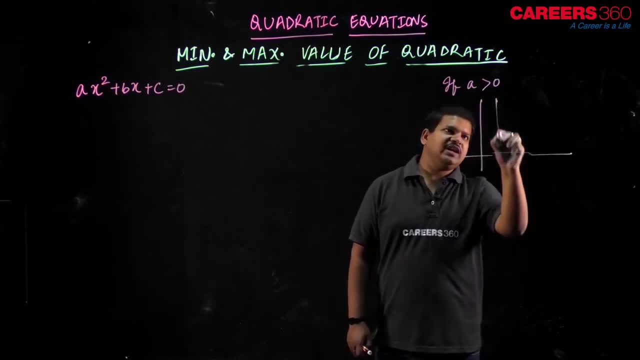 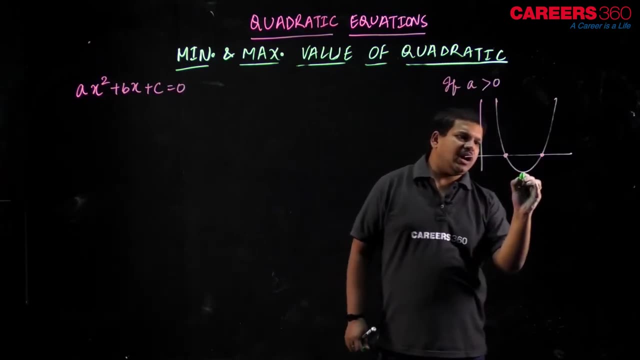 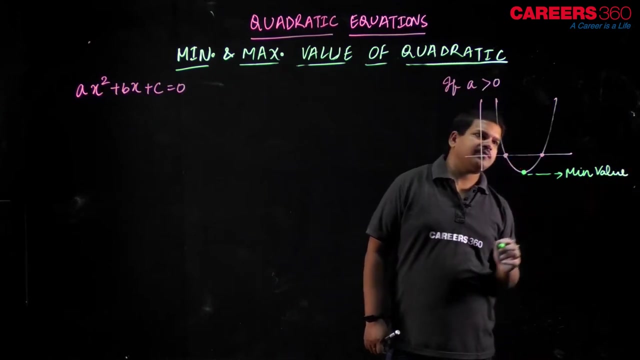 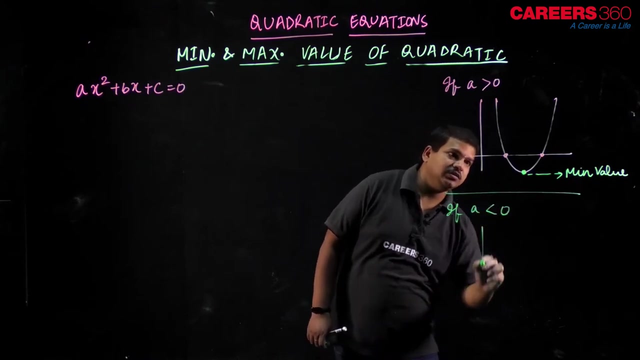 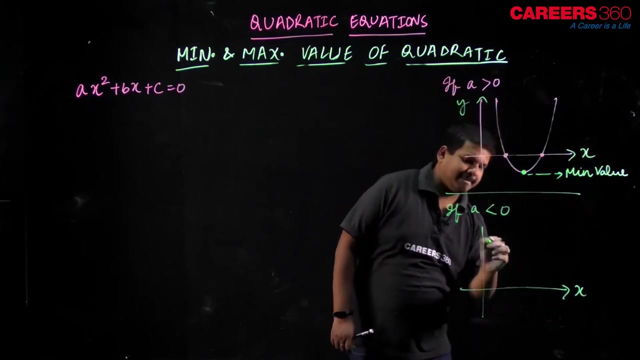 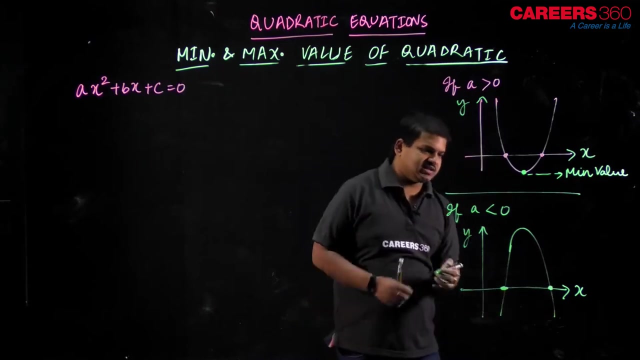 A is greater than 0, then the graph will be looking like somewhat like this: right, there will be two values and at this point, there, this will be the minimum value. occur right Now. what if? if a is less than 0, then in that case the graph will look somewhat like this and in this case this will: 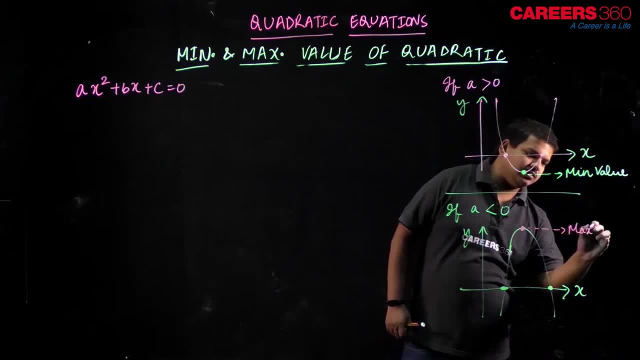 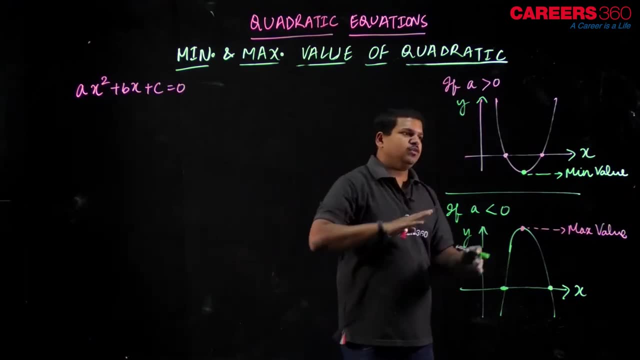 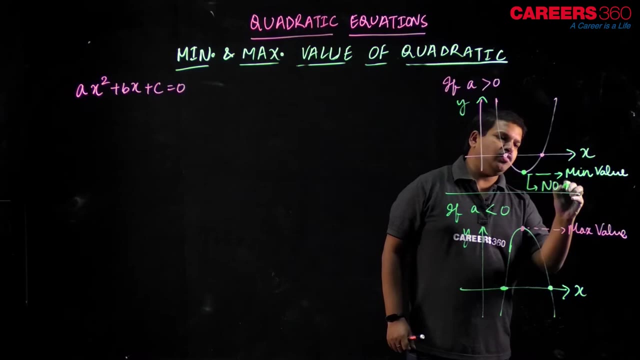 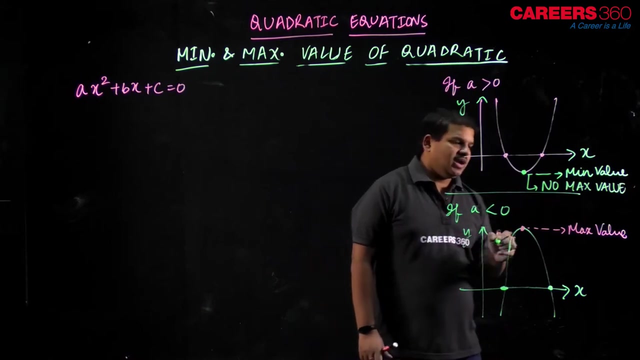 be the maximum value of the quadratic. right Now, you need to understand one thing: if a is greater than 0, minimum value will occur at a greater than 0. At this point, and there will be no maximum value, there will be no maximum value. and if 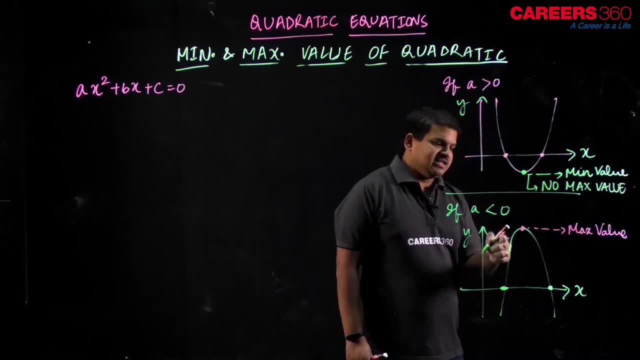 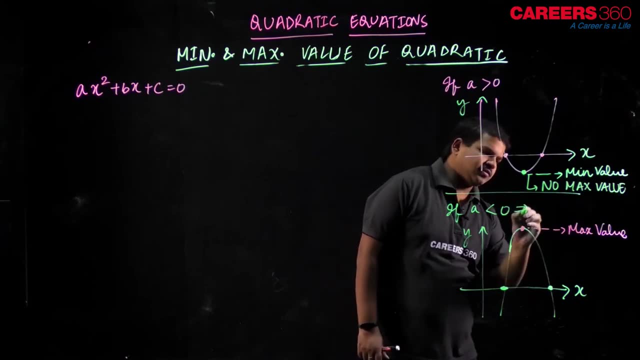 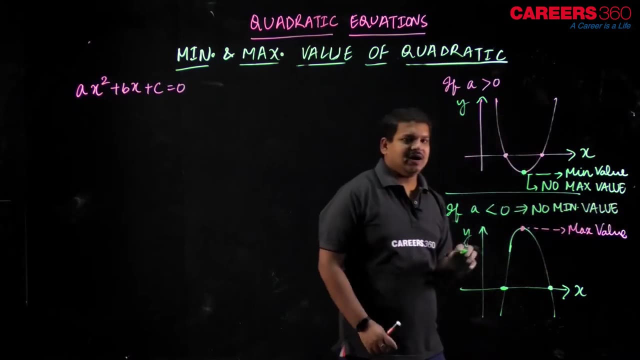 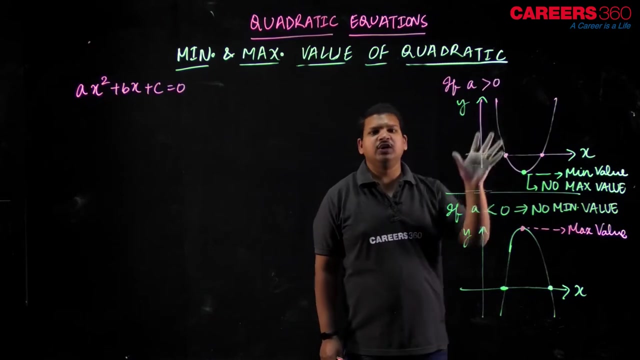 a is less than 0, then this point will be the maximum value point and in this case no minimum value will occur, right? This should be very clear to you, right? because some students gets confused that this is tending to infinity. no, this is not tending to infinity, this is simply we. 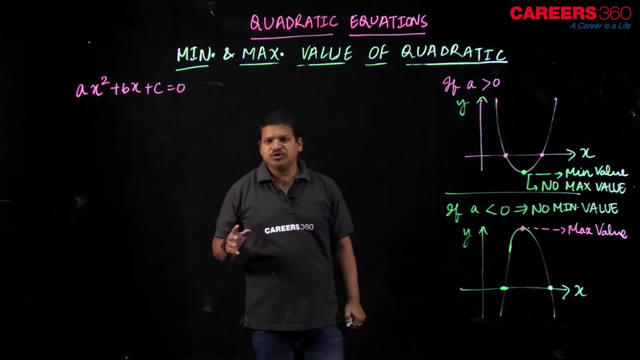 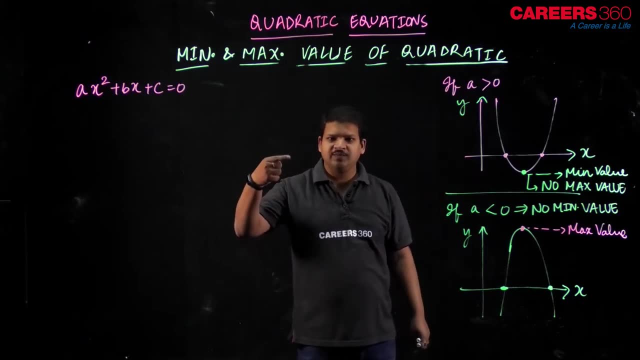 don't have any maximum value. see. so, if there is a option in which there is a first option says find out the maximum value in this case, and first option is given no maximum value, second option is given infinite maximum value. So you will put first one, correct? 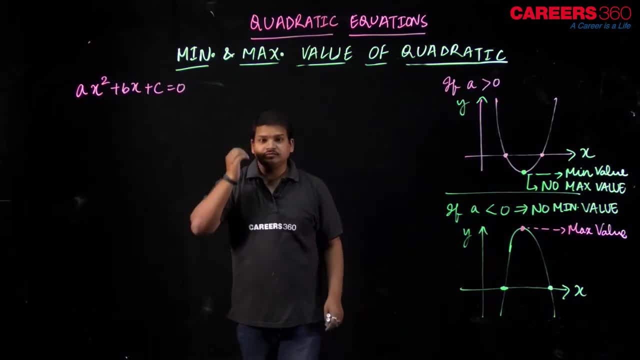 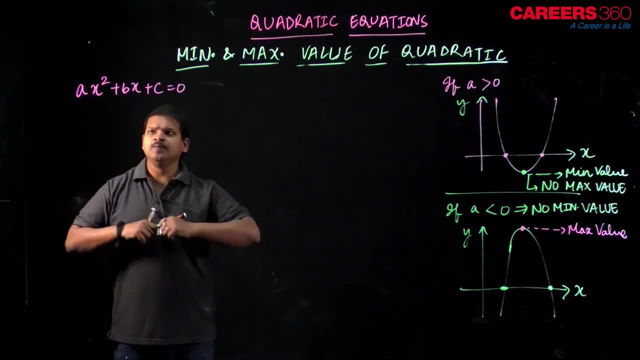 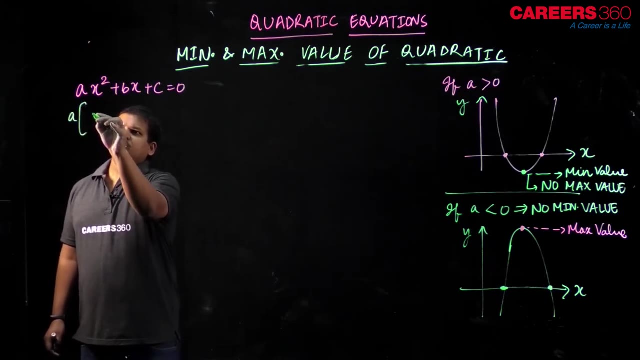 I hope it is making sense to you right now, proceeding towards our mathematical derivation of this minimum or maximum value, all you need to do is just to rearrange this thing a bit. let us take a common out of it. So what I will be remaining with is b upon a. x plus c is equals to 0, and if I do a bit, 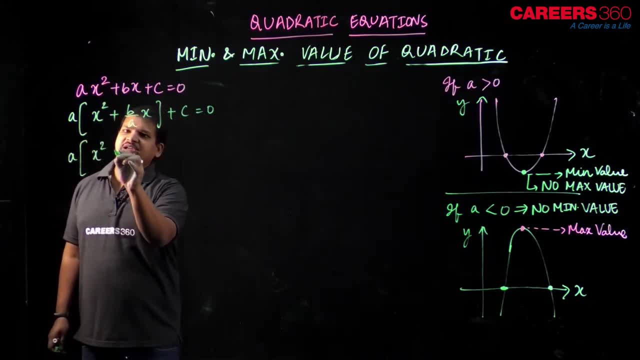 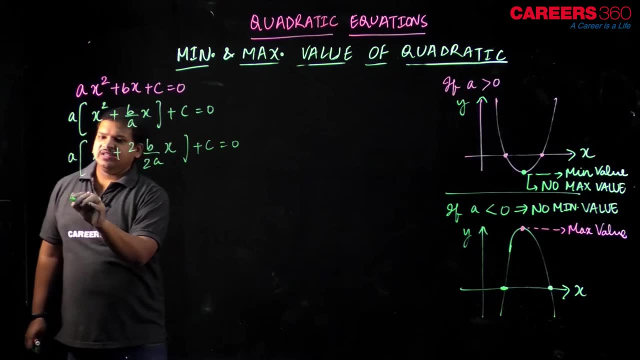 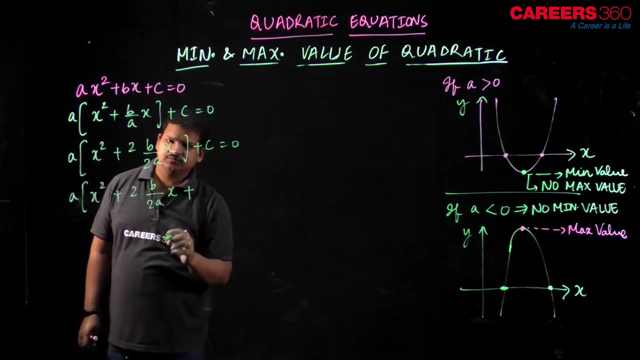 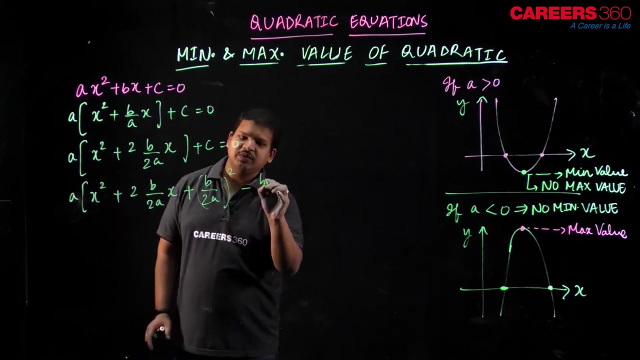 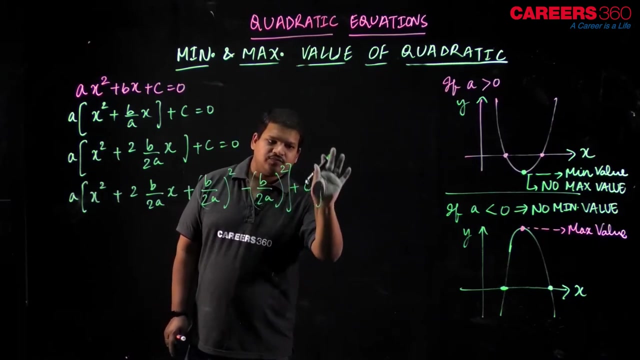 of rearrangement. Let us say and divide 2 a in the middle term, and then I am adding, I am adding ah, b upon 2 a whole square. if I have added, then I have to subtract b upon 2 a whole square as well. plus c equals. 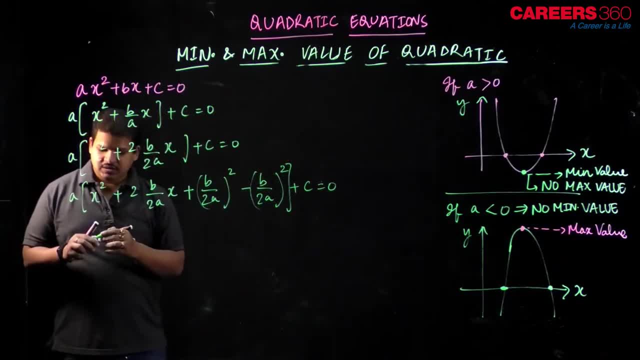 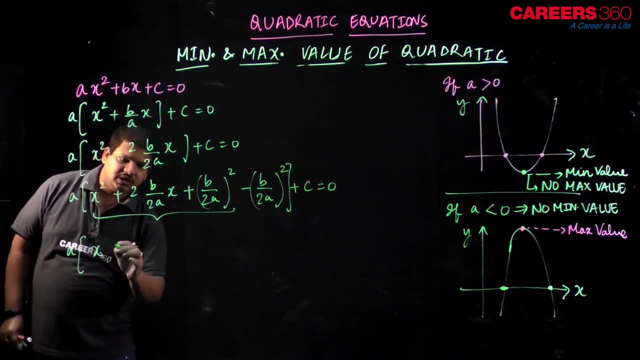 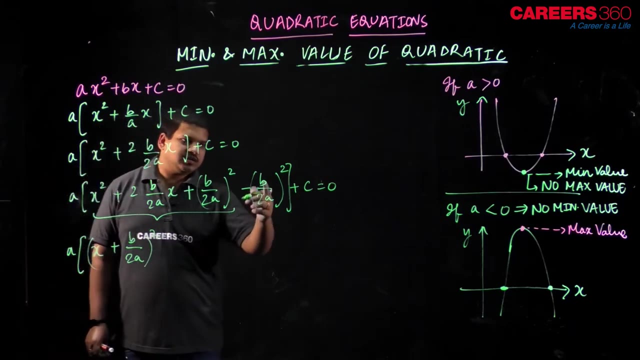 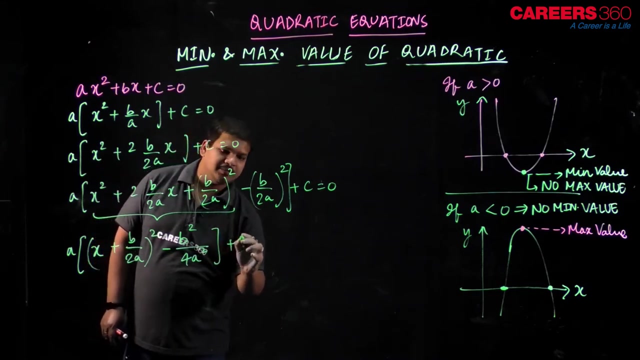 to 0 and again, if I see this will become what this is: x plus b upon 2, a whole square right, and this will be b square upon 4. a square plus c is equals to 0, and if I open the bracket, so I will be remaining way. 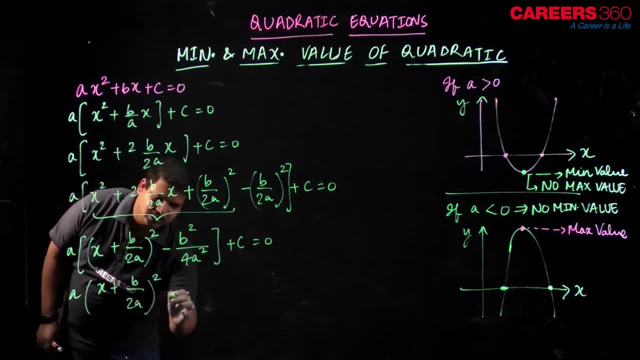 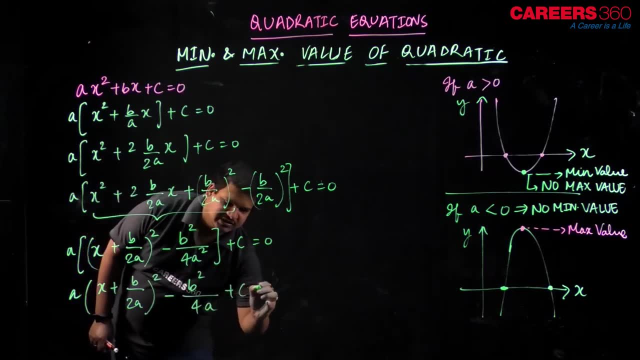 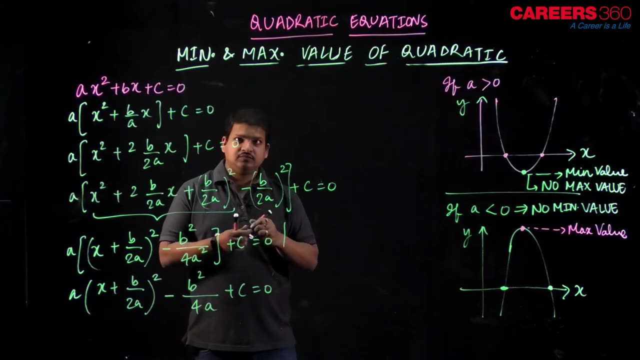 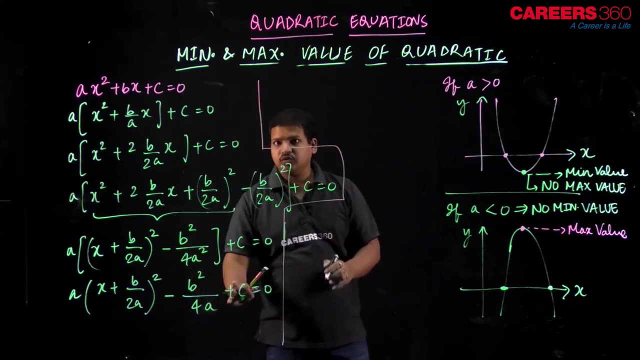 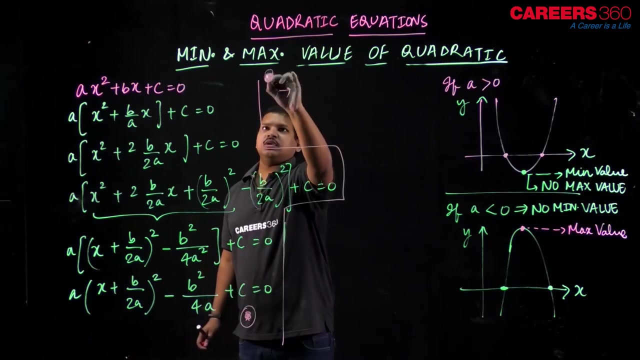 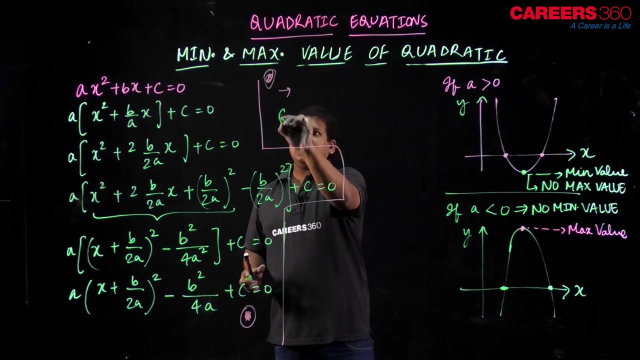 With x plus b upon 2, a whole square, and then minus of b square upon 4, a plus c is equals to 0, and let us draw some lines over here. right Now, what I am going to do is continue from here. nothing else. nothing is continued from here. So next step would be A into x plus b upon 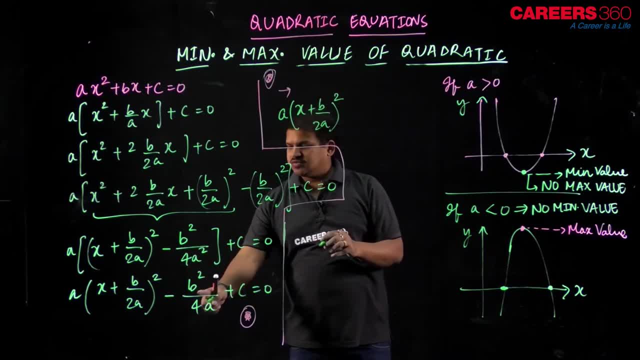 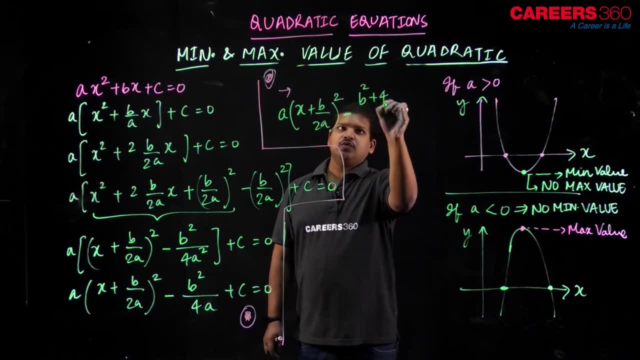 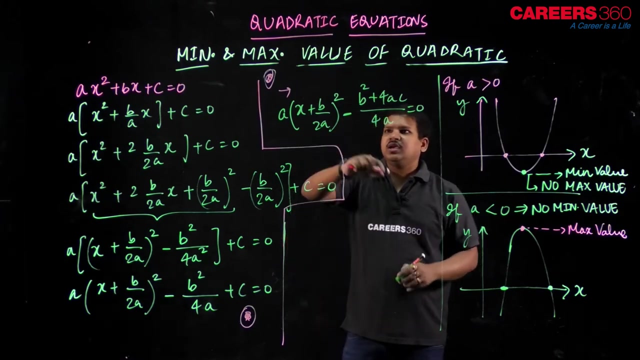 2 a whole square. Now this would be what b minus of b square plus 4 a c upon 4 a Right, iva, right, and this is equals to 0.. Now you have to understand one thing: that if in this equation 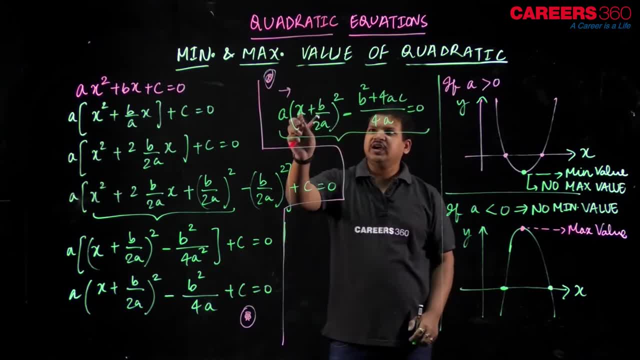 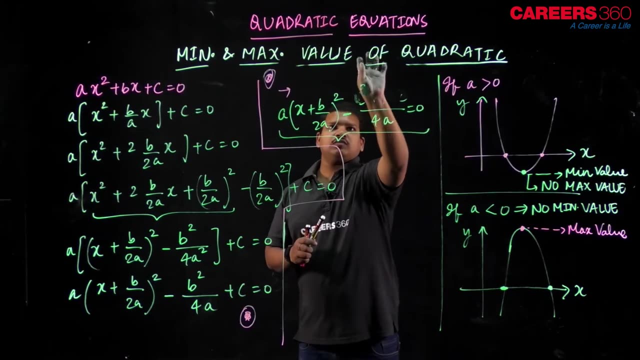 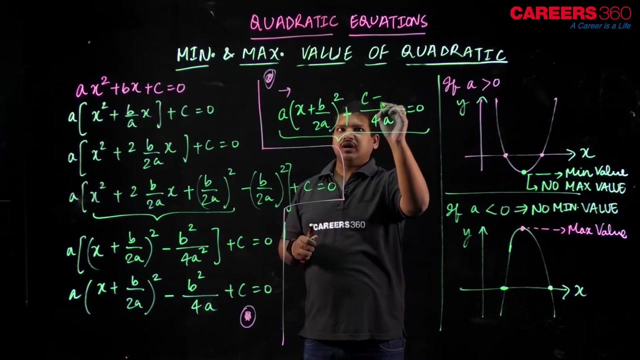 if in this equation I put to get the minimum or maximum value, both the values I am talking about. right, if I need to get minimum or maximum value, let us rewrite it as. let us rewrite it as c minus, see 4 a c. 4 a c minus b square. right, yes, 4 a c minus b square. this would 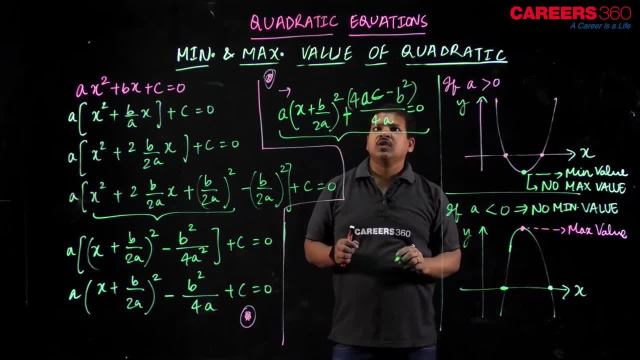 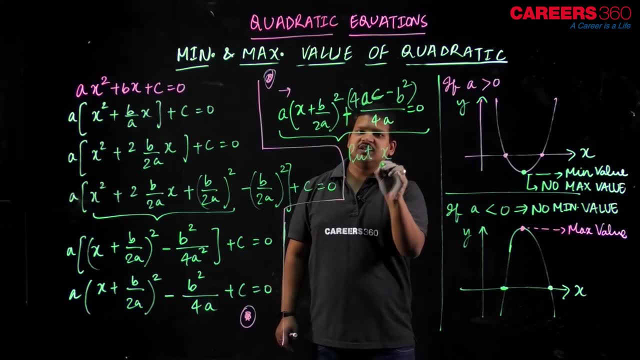 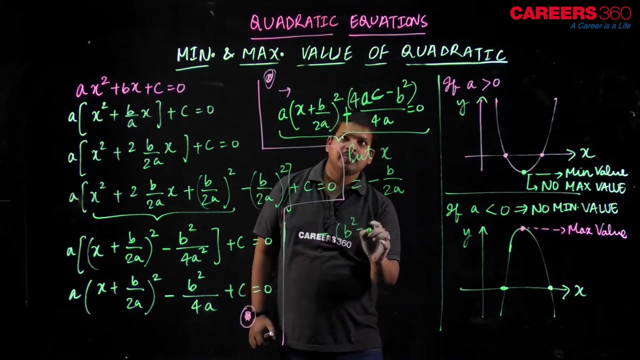 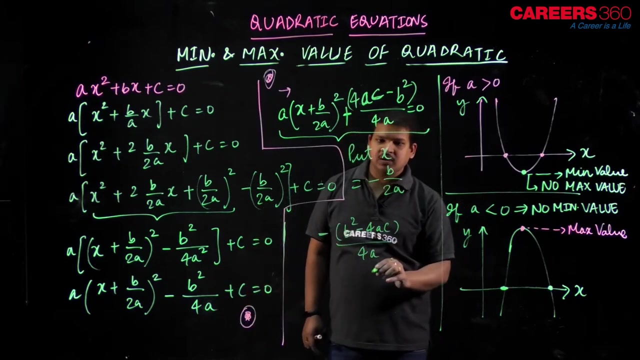 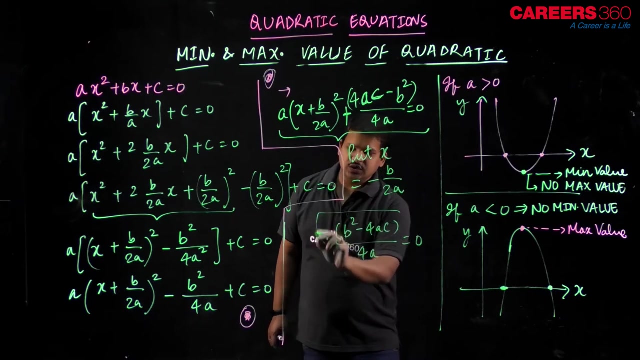 be more Better representation. all right Now, if I put x equals to minus b upon 2 a, in this particular value, I will be remaining with minus of b square minus 4 a c upon 4 a, right union 7.. And this is equals to 0.. So see this value, this value will be the minimum. 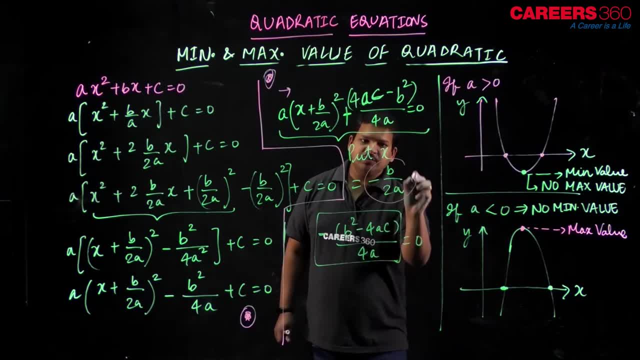 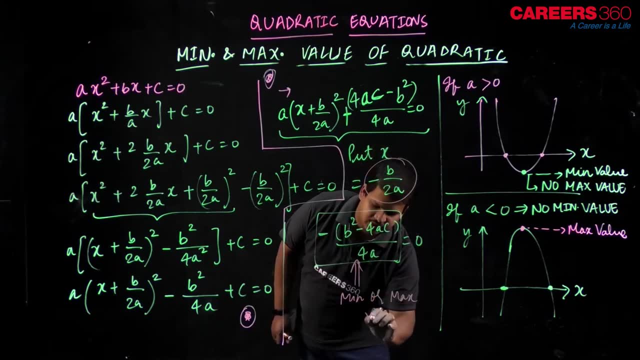 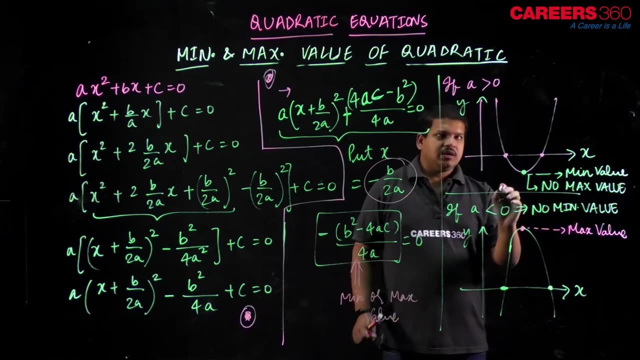 or maximum value of the quadratic. So at b is equals to 2, a. this will be minimum or maximum value of a. quadiziохusithe constraint mechanics. again, we will see both conditions. If a is greater than 0, then at this value is what This value will be minus b upon 2a. 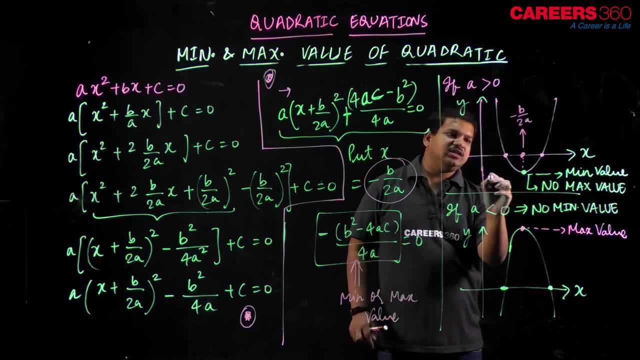 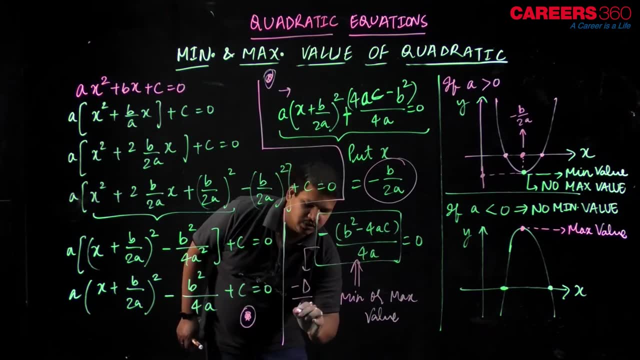 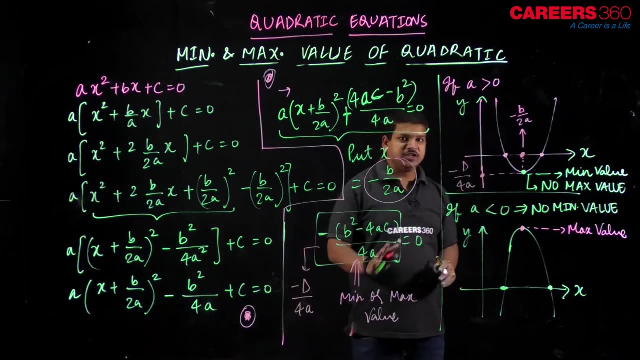 This will be minus b upon 2a and this value will be what? This? I can write it as minus of d upon 4a, So this value minus of d upon 4a. I hope it is making sense, because this is what This is, y, or I can say this is fx. 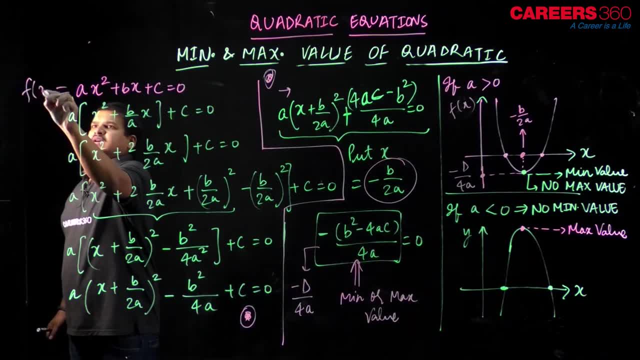 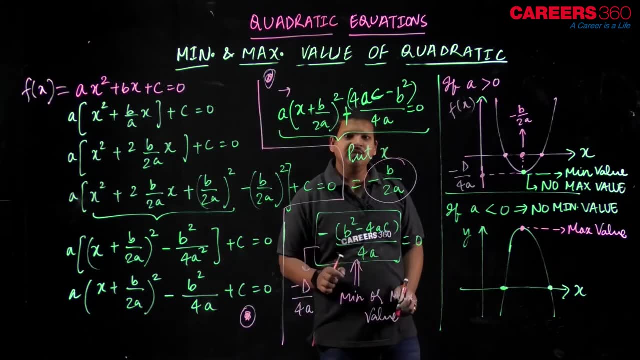 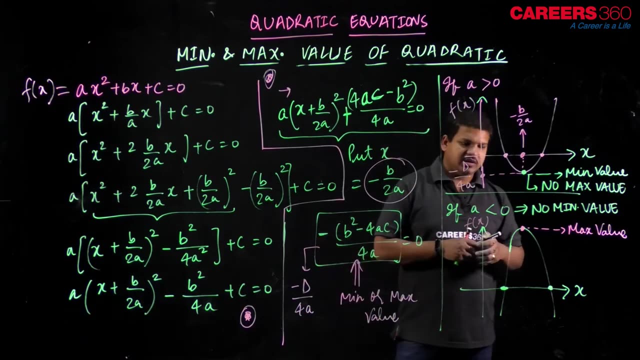 Right, This is fx, Right. So the value of fx is what Minus of d upon 4a? Again, let us make it fx as well. Make this fx as well, Right? So again, this value.